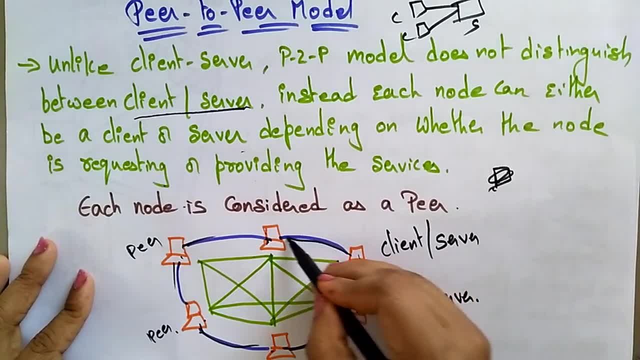 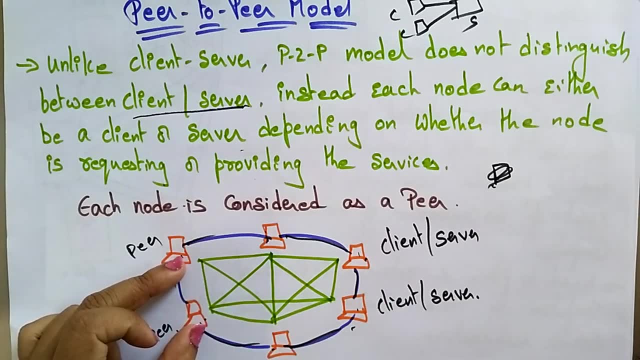 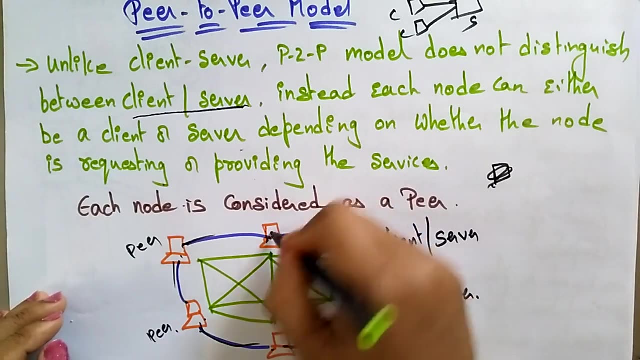 to the network, So all are connected in the network. And now these systems, how they are going to be communicated Based on the requirement. Okay, So this system can request and this system, as well as it, can reply, because this, each system can, acts as server as well as a client. That is a. 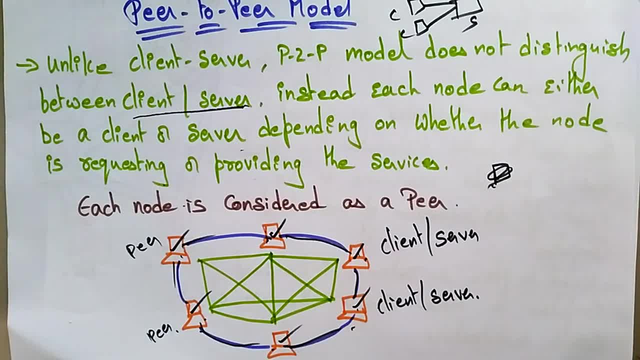 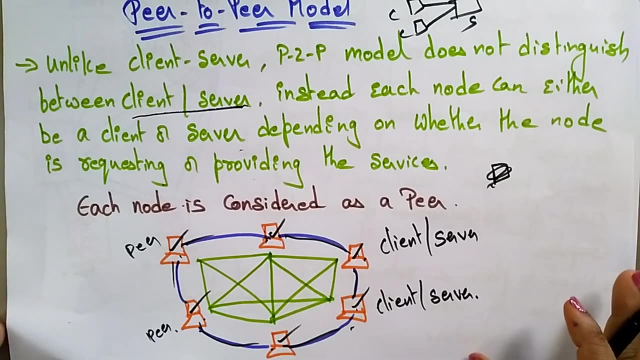 peer-to-peer model. Instead, each node can either be a client or a server, depending on whether the node is requesting or providing the service. Suppose it is requesting, means it can be a client. Suppose it is responding, means it is, it may be act as a server. So this is an architecture. 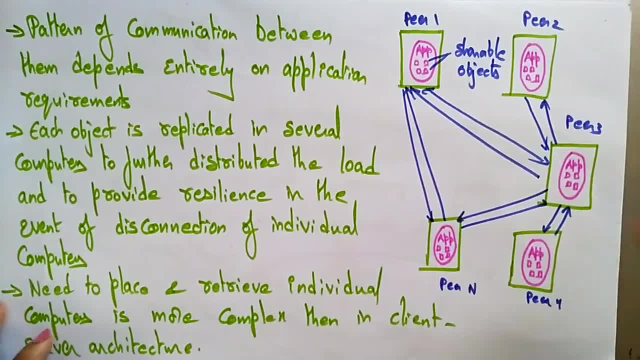 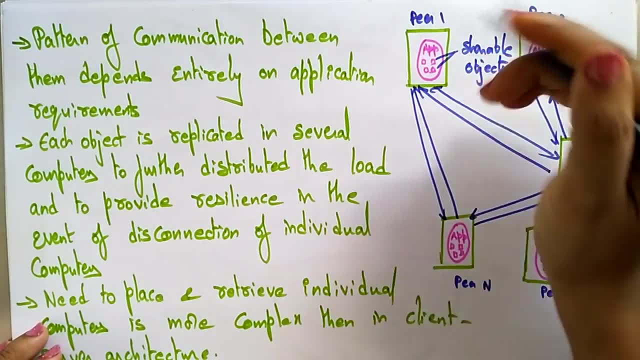 of the peer-to-peer model. Let me show you here. So peer-to-peer means different systems are there. Let me take N. systems are present in the network. This system is having their applications, their own applications. That application is having those objects, different objects. 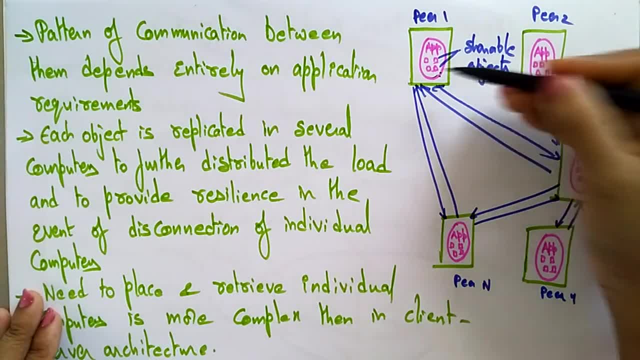 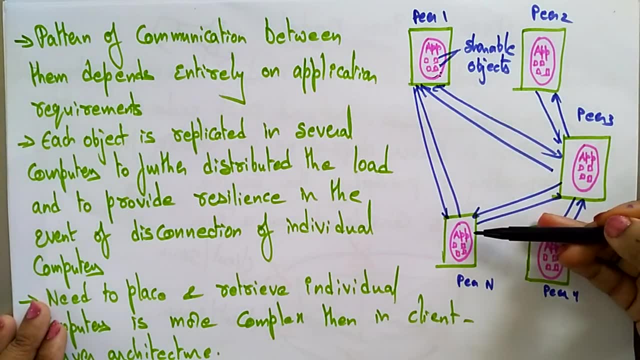 Even those objects can be shareable. Those objects are shareable Means the peer-to-peer system. objects can share by peer-to-peer and the peer-to-peer can share the objects to peer-to-peer. and here the peer-to-peer can share to peer-to-peer. 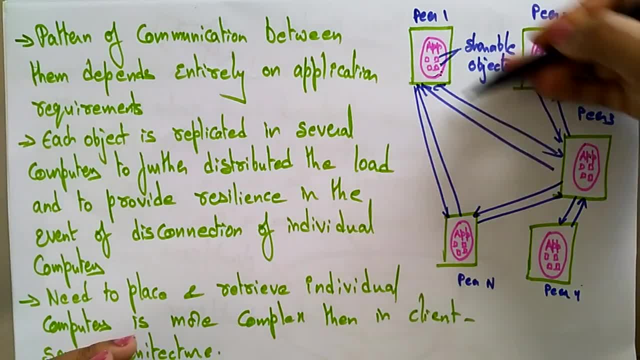 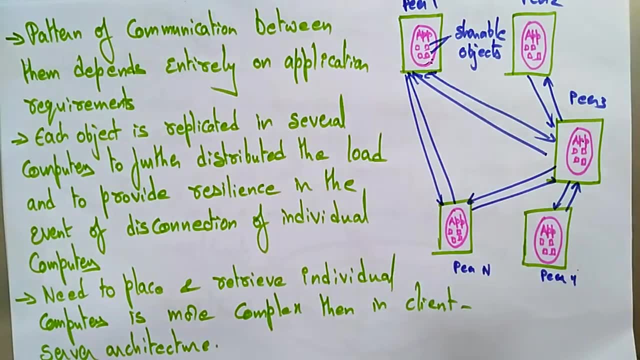 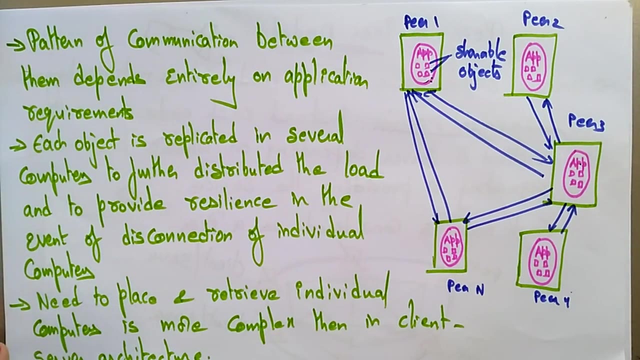 to means like anything. so whenever it is sharing, it becomes a server. the other becomes the client. whenever it is, uh, this system is sharing, it becomes a server and this becomes a client. okay, so each system can access a client as well as server in the peer-to-peer model. so let's see. 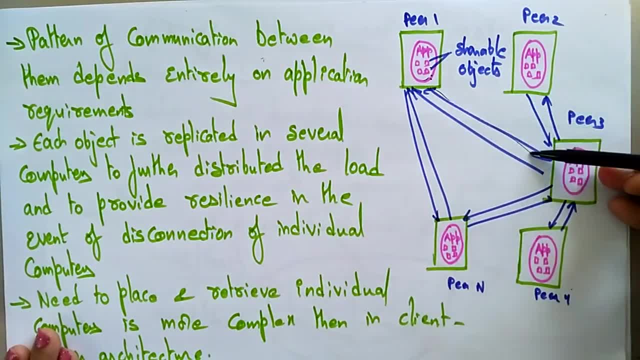 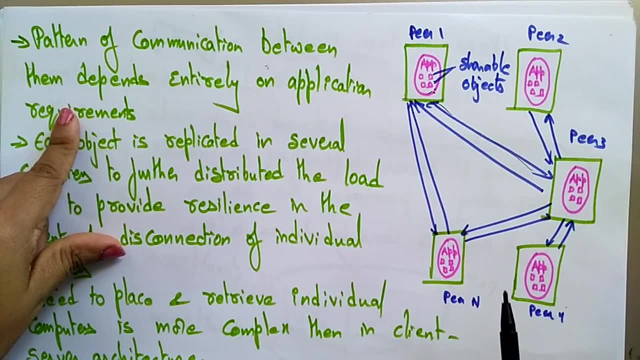 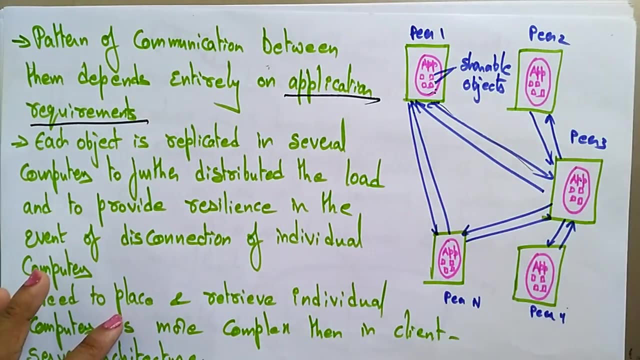 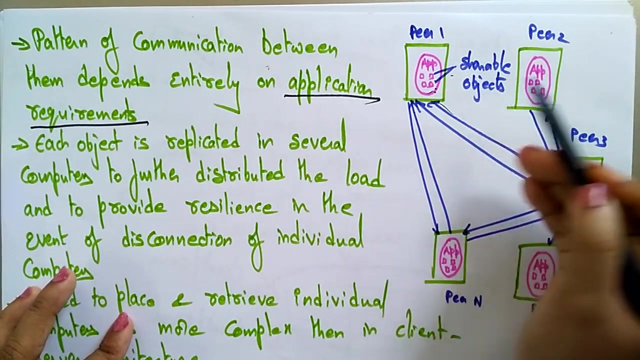 the pattern of communication. so here this is. did you see, this pattern of communication, this pattern of communication between the systems depends entirely on application requirements. so it's this pattern, this type of communication is completely, entirely depends on application requirement. so here, did you observe these two systems are not connected. why it is not connected? 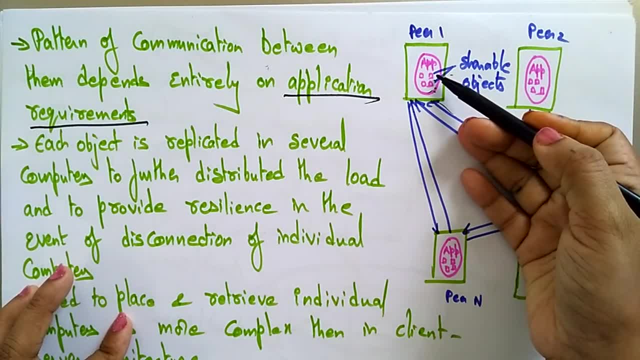 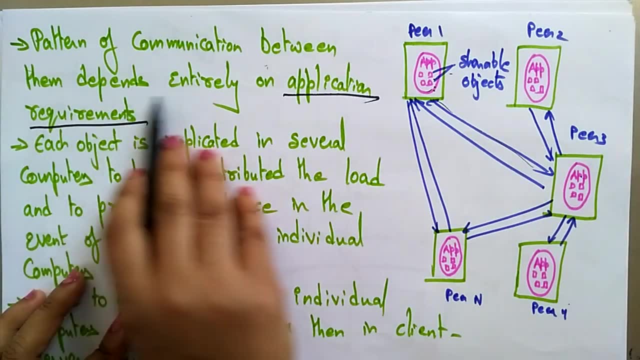 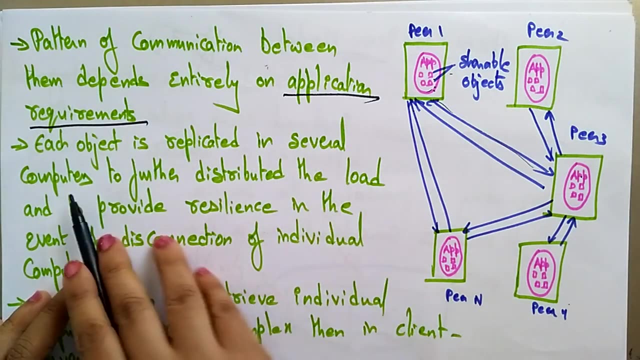 because they did. this system don't want the objects of this system and this system don't wants the object of this system, so that's why the pattern of communication between them depends entirely on application requirements. Each object is replicated in several computers to further distribute the load and to provide resilience.